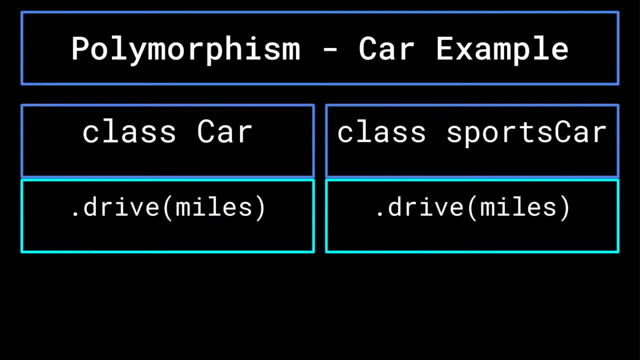 representing the number of miles you would like the car to drive, and the car's gas attribute will be decreased by the pertinent amount In the car class. you may create a sports car class. The dot drive function may cause the car's gas to decrease by 0.04. 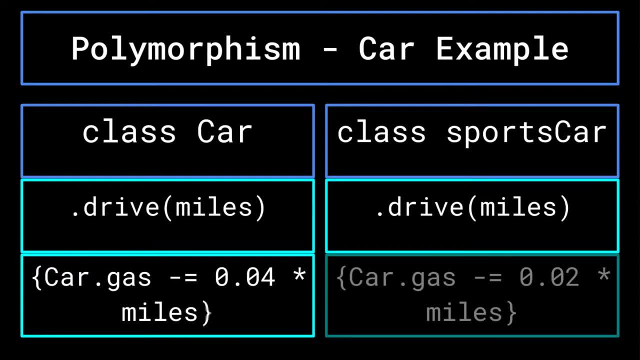 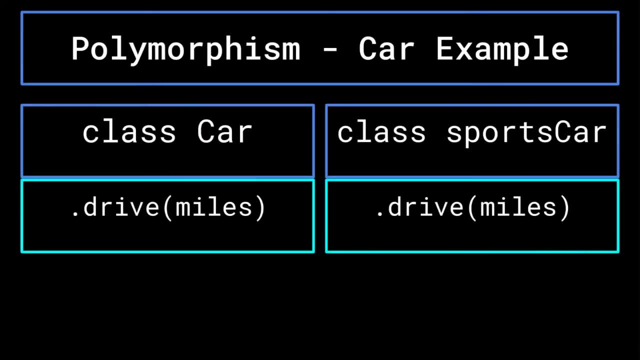 gallons per mile, whereas the sports car class may instead have its gas decreased by 0.02 gallons per mile. If you create an instance of a sports car called mySportsCar, the sports car implementation of the dot drive method will override the generic car version of the. 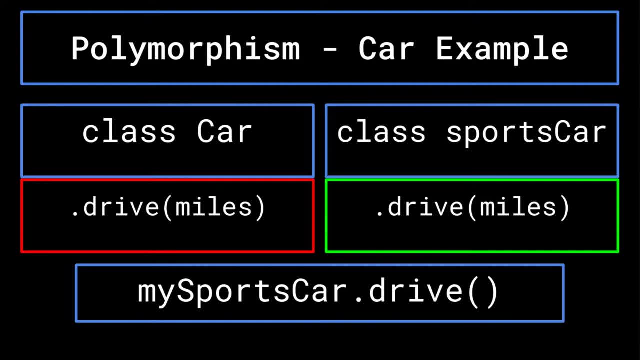 dot drive method. Therefore, mySportsCardrive will decrease mySportsCar's gas attribute by 0.04 gallons per mile. If you create an instance of a sports car called mySportsCar, the sports car implementation of the dot drive method will override the generic car version. 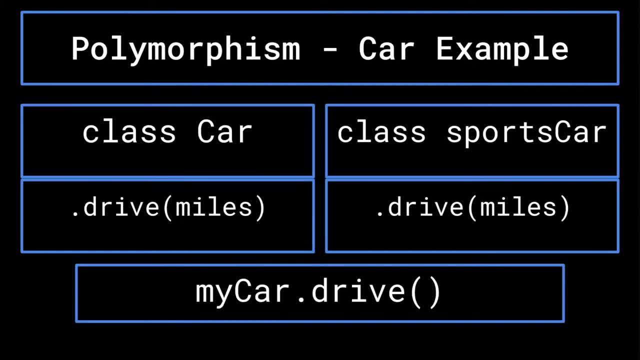 of the dot drive method. Therefore, mySportsCardrive will decrease mySportsCar's gas attribute by 0.02 gallons per mile. However, were you to create an instance of the car class called myCar, myCardrive would instead decrease myCar's gas by 0.04 gallons per mile. This 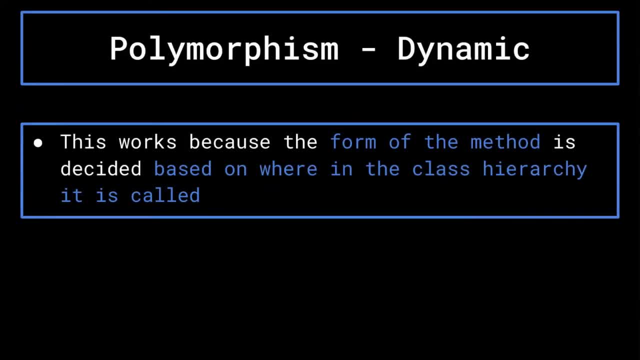 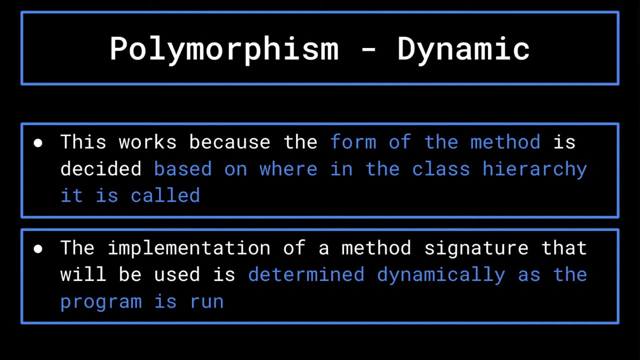 is an example of dynamic polymorphism, as the implementation of a method signature can change depending on which level in the class hierarchy that it is called. This works this way because the form of the method that is called is decided dynamically as the program is run. This idea can be extended across a class hierarchy in more layers than just. 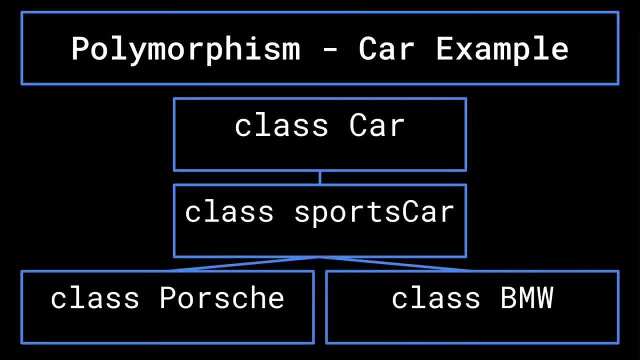 two. You could add more subclasses representing different types of sports cars with their own dot drive methods with different implementations, and creating an instance of each of these subclasses would use their own implementation of the dot drive method when called. The main benefit of dynamic polymorphism is that it allows you to write methods in the superclass. 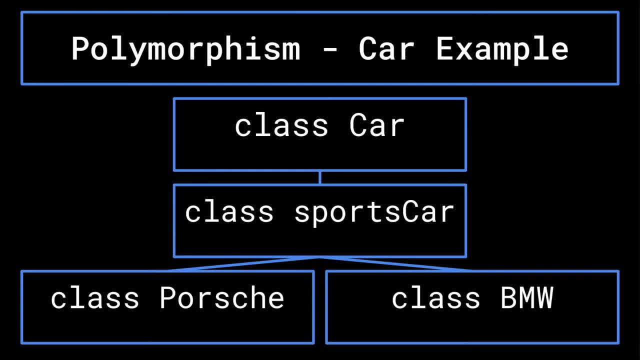 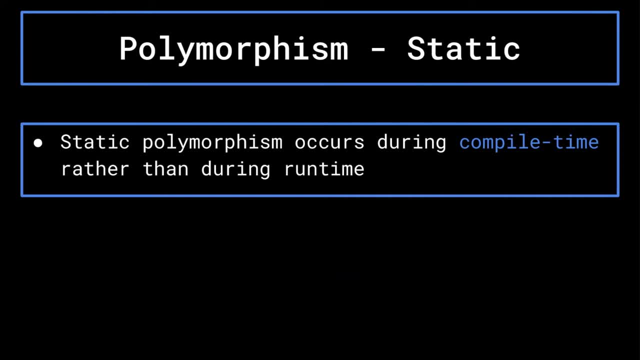 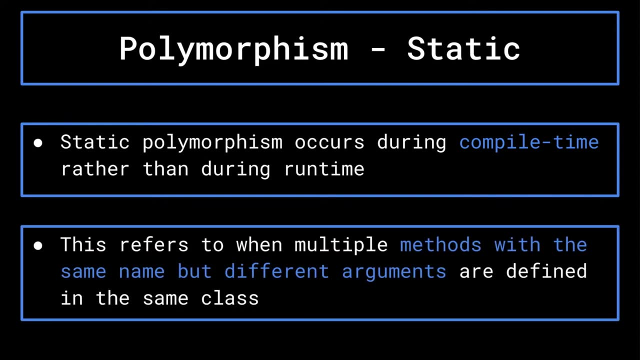 without having to include ifs and else ifs to account for exactly which subclass is being used. The second type of polymorphism is static polymorphism. Static polymorphism occurs during compile time rather than runtime. This refers to when multiple methods with the same name are defined in the same class. In this case, the methods are differentiated by their 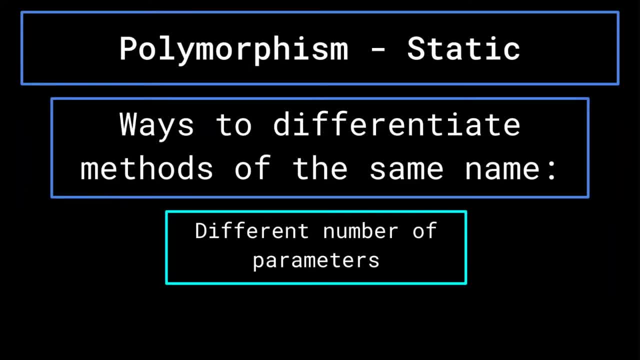 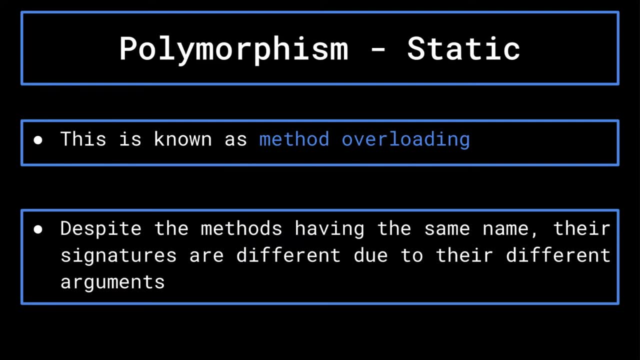 arguments. Either they take a different number of parameters, they take parameters of different types, or they take parameters in a different order than one another. This is known as method overloading. Despite the names of the methods being the same, they have different method signatures due to their differences in the 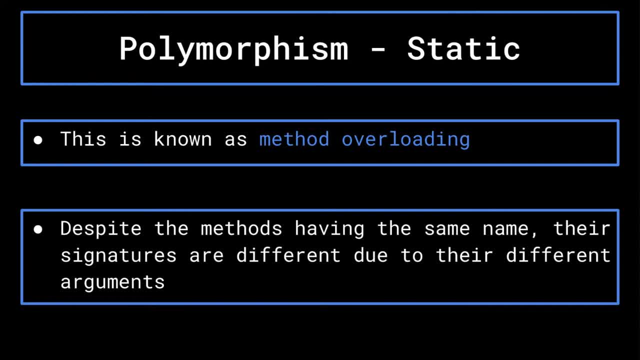 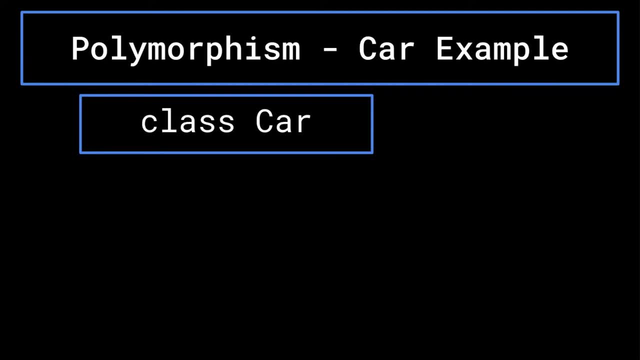 parameters that they accept. To better understand this, let's go back to the car example. Let's say that you are working in the car class. In this class, you are looking to create three different drive methods. The first drive method's argument accepts one integer and. 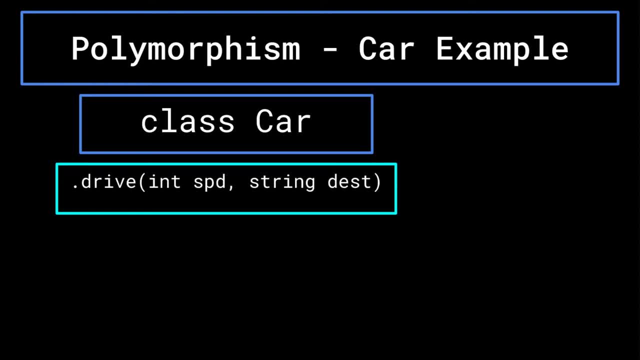 one string as parameters, say speed and destination. For clarity, we will refer to this one as drive method 1, however, keep in mind that its method name is just drive. For drive method 2, we will set its argument to accept two integers, for instance distance and speed. 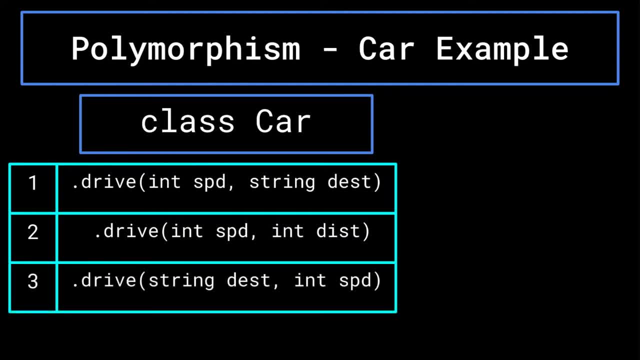 Finally, in drive method 3, we will have it accept a string first for its destination and then an integer for speed. This differs from drive method 1 in that drive method 1's parameters are in reverse order compared to drive method 3.. In each of these three example methods, the method signature: 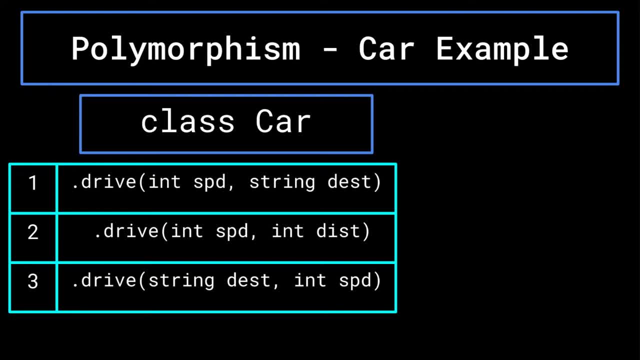 is different despite the methods having the same name. Therefore, the computer is able to tell the methods apart when the program is being compiled. For example, were I to call mycardrive 45 work, drive, method 1 would be called, as the argument given indicates. 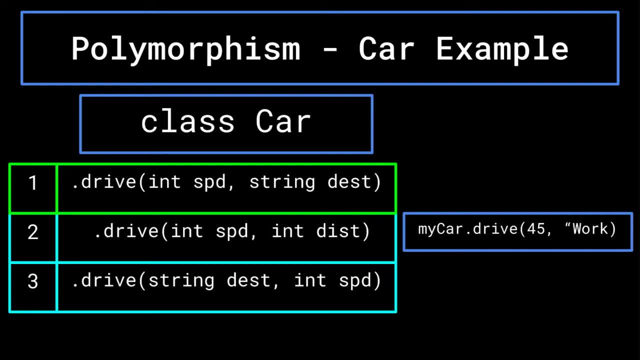 that this is the method I would like to call. Furthermore, mycardrive 15- 60 would call drive method 2, and mycardrive school- 30 would call drive method 3.. When implementing method overloading, the different methods tend to have separate but similar effects. 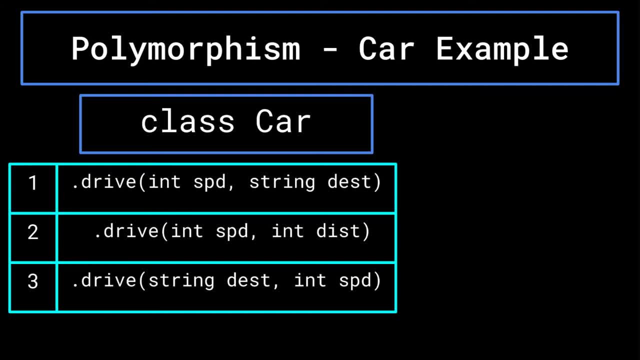 Despite drive method 1 and drive method 3 being the same method, the method overloading is not the same method as the method overloading method 1 and the method overloading method 3. taking the same parameters, it is likely that their implementation would be different. 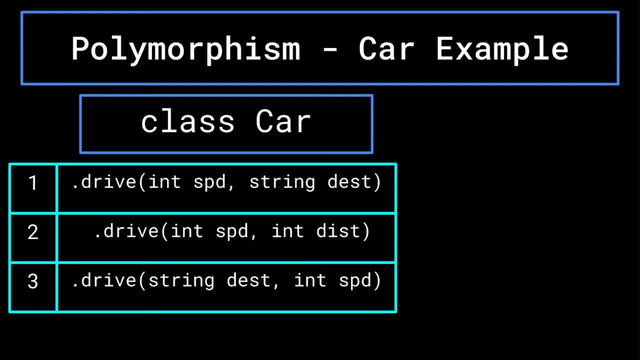 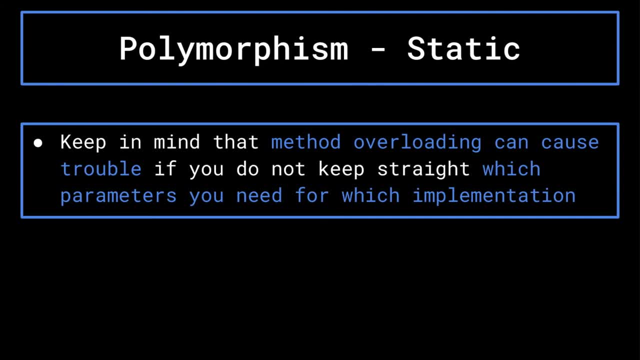 and thus would achieve separate effects. Otherwise, there would be no reason to have both methods. Keep in mind that method overloading can cause trouble if you do not keep straight which of the method's implementations you would like to execute and what form of argument.